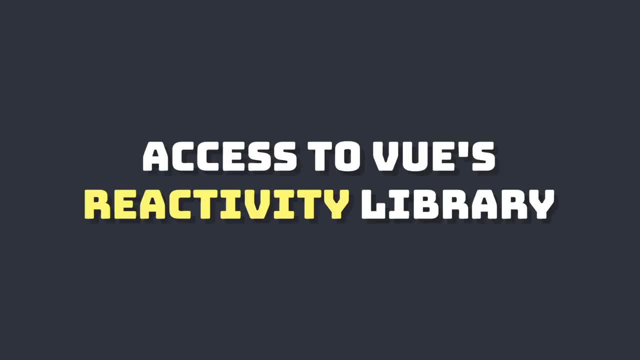 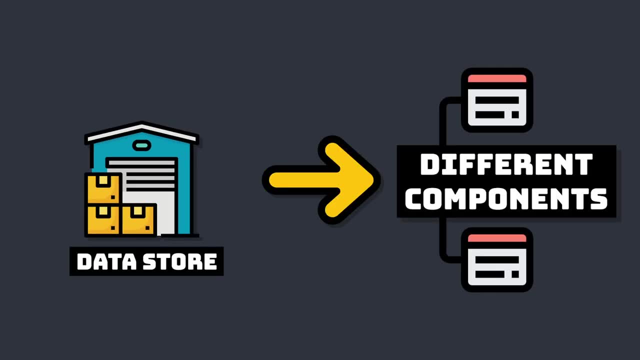 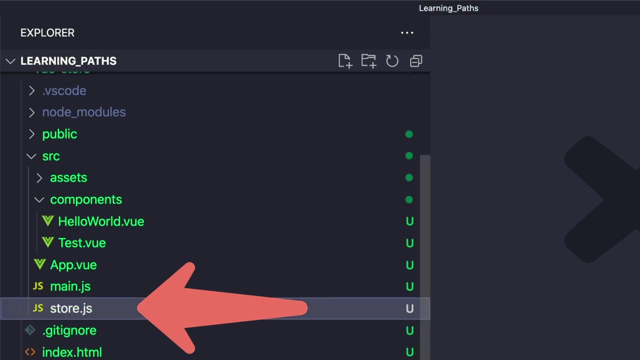 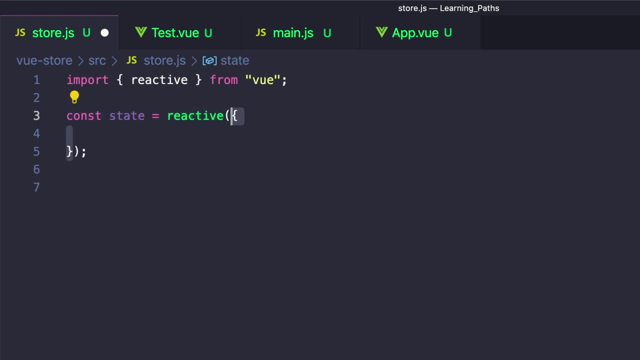 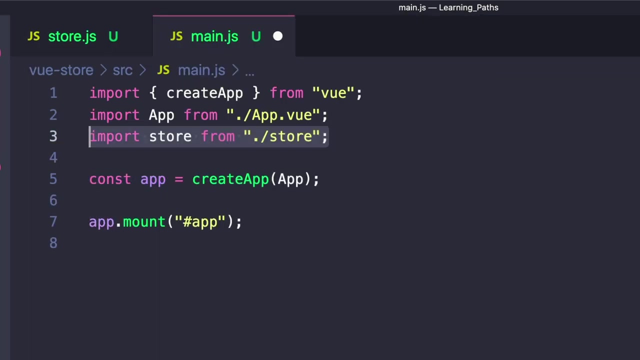 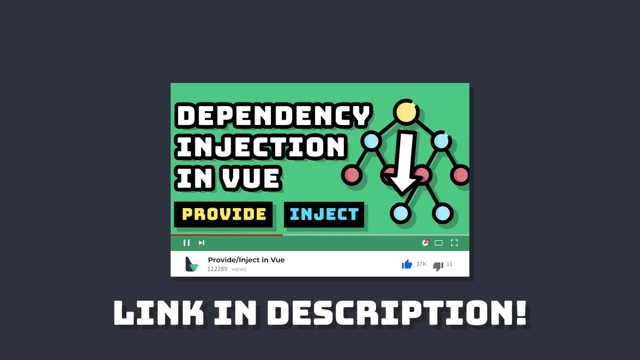 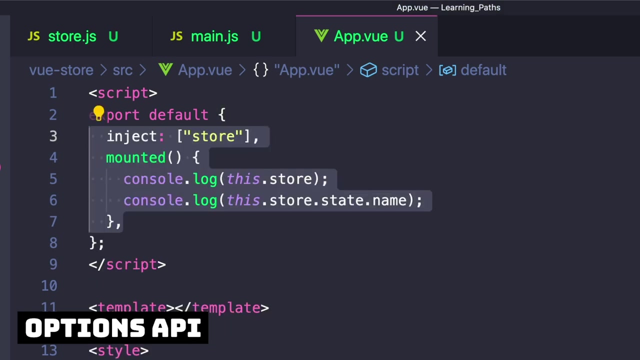 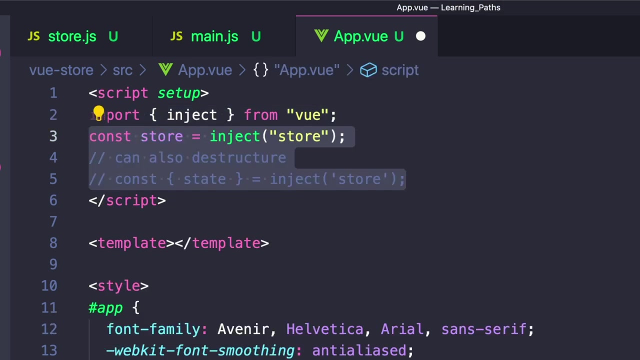 Vue 3 gives us developers access to Vue's reactivity library. And one cool thing we can do with this is create our own data store that we can use to create different sources of truth across our app. And as you can see by the length of this video, it's incredibly easy. So to set up our store, let's create a file called store.js inside of our source folder and import reactive from Vue. To create our state, we can create a constant called state and set it to a reactive object. And for now, let's just say name. And then all we have to do here is export our state. Then if we want to use our store, we can go to main.js, import our store, and then call app.provide and pass in our store. And if you want to learn more about the provide inject syntax, check out this video in the description. And then inside any component, we can inject our store in either the options API by defining an inject property and then passing in store or in the composition API where we import inject from Vue and then set a constant store to inject store. Then in our template, we can access our state and then our name property. And that's it. We have a basic flow of our data store. 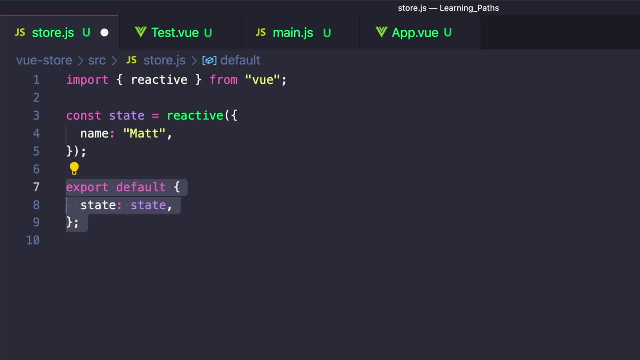 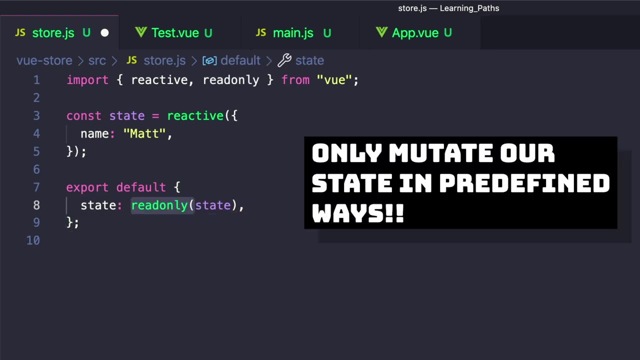 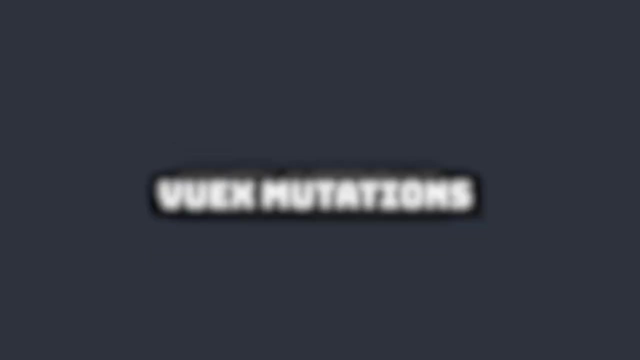 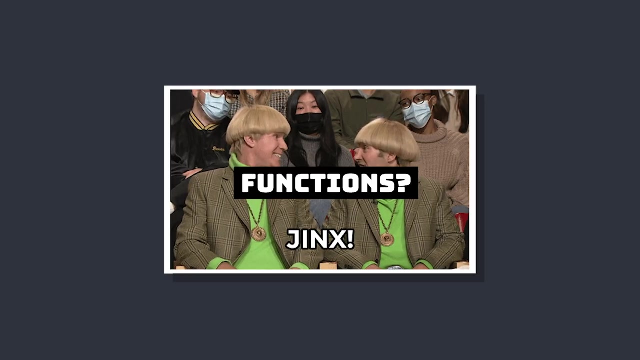 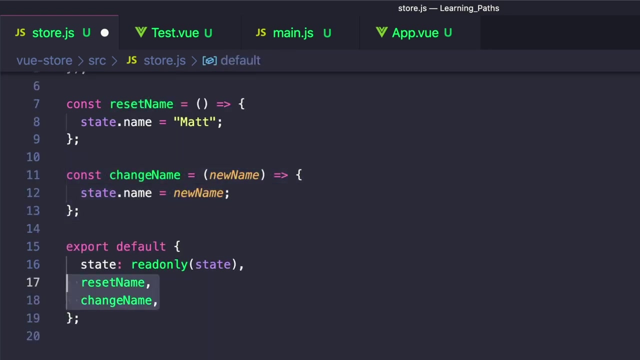 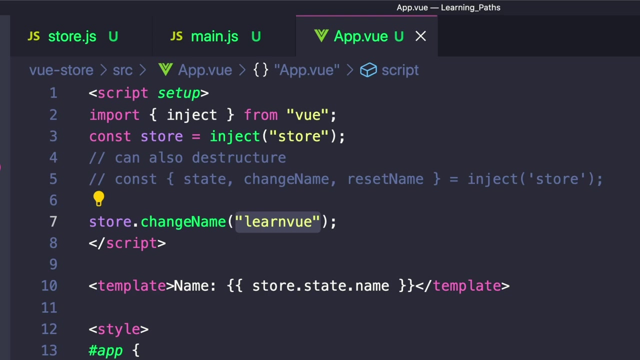 But let's go back to store.js and make this a little bit more legit. And one great practice is to return a read-only value of our state. This is similar to VueX mutations, where we only change our state in predictable ways. And these ways are similar to actions and mutations. In our custom store, the concepts of actions and mutations will be merged into one. While you can create your own naming conventions that follow VueX or Pena more closely, in our example, both are functions, so there's no real distinguishing between them. So let's create a function that resets our state to mat and then a constant that changes our name to a new value. We'll add these to our export default. Then inside of our Vue component, we can call store.changeName or store.resetState, just like we would in any other data store. As always, there are pros and cons to this.